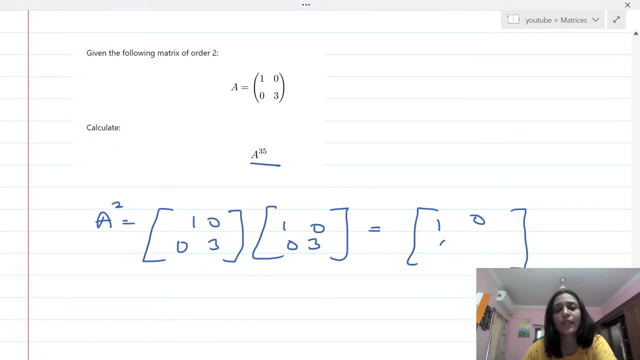 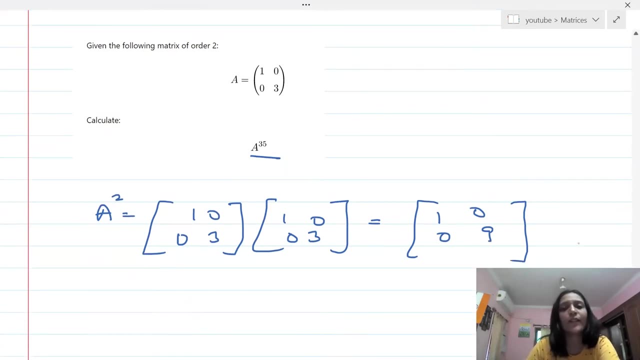 and then I have 0 into 1 is 0, 3 into 0 is 0, and then I have 0 into 0, which is 0, and 3 into 3, which is 9.. So the square we are getting as 1009.. Let's find out now what a to the power 4 would be, which is. 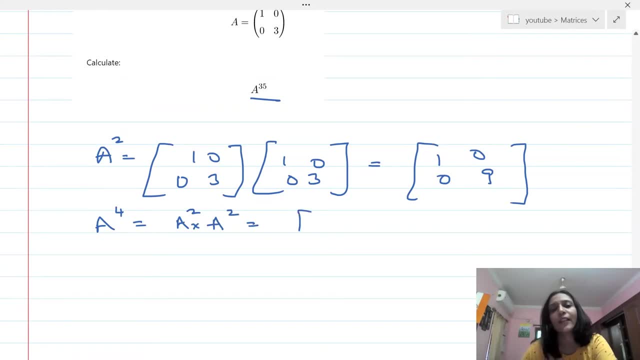 nothing but a square times a square. This is going to be 1009 times 1009, and the key thing that you should see over here is: I'm trying to figure out a way in which I can get some type of pattern, So 1009 is going to be: 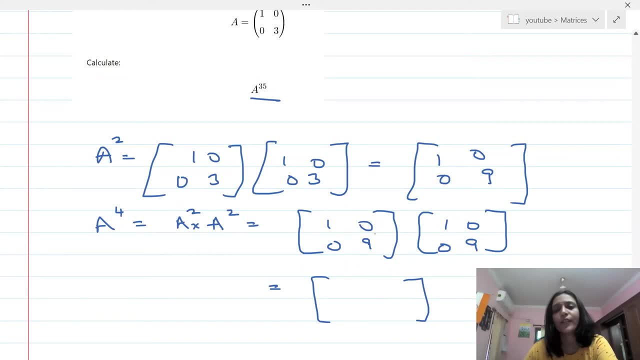 1009 times 1009.. 1 into 0 is 1, 0 into 0 is 0, so this will be 1.. 1 into 0 is 0, 0 into 9 will be 0, 0 and 0 again. 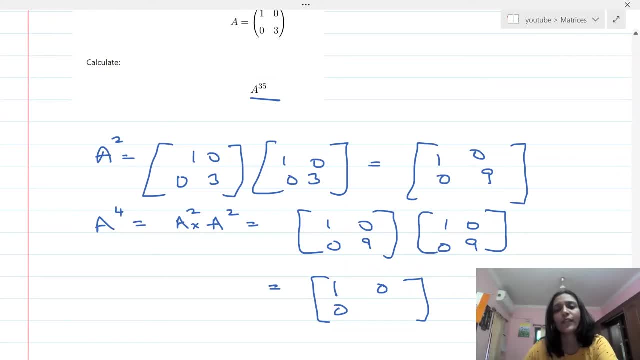 and then 0 into 0 is 0 and 9 into 9 is 81. So if one thing you observe is that, as whatever the power of a is, that becomes the power of 3 over here. So if this is to the power of 4, this is. 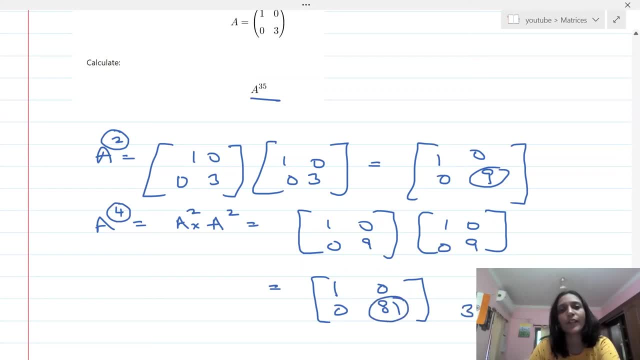 becoming 81, which is 3 to the power of 3.. So if this is to the power of 4, this is becoming 81, which is 3 to the power of 4.. So with this, can anyone guess what a to the power 35 is? I'll just give you 10 seconds. 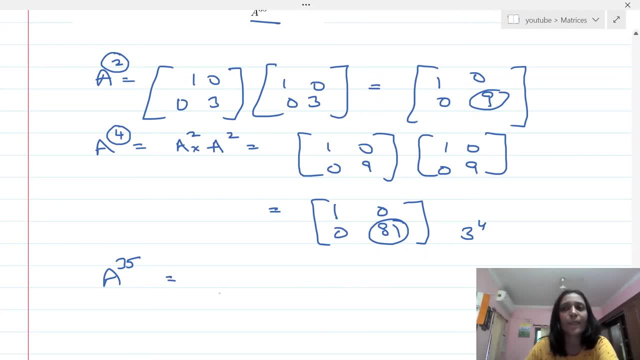 Pause the video. try to solve it All right. so that's right. the answer should be 1003 to the power 35.. That should be your answer. So like this, we can find out the answers of any matrix to the power n by figuring out what the pattern is, by first finding a square a to the power 4 and some or 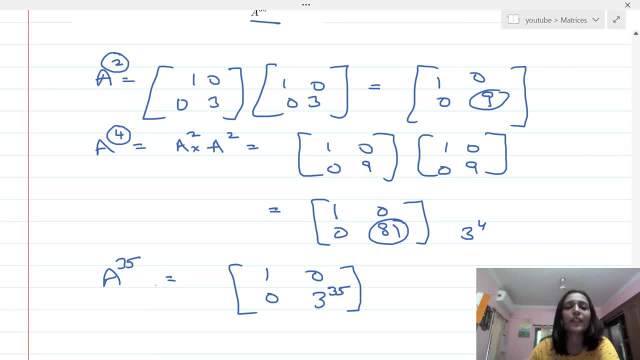 the other pattern will emerge, and then you would be able to successfully solve the question. I hope this video helps. Do hit the subscribe button and like and comment for more. Thank you.